say that if two or more lines are cut by a transversal and corresponding angles a congruent, then the lines are parallel. okay, so now that we know that the lines are parallel, let's label them in the diagram. and now here's the reason: why is it that these segments are congruent? what justifies this? so let me label the steps. so 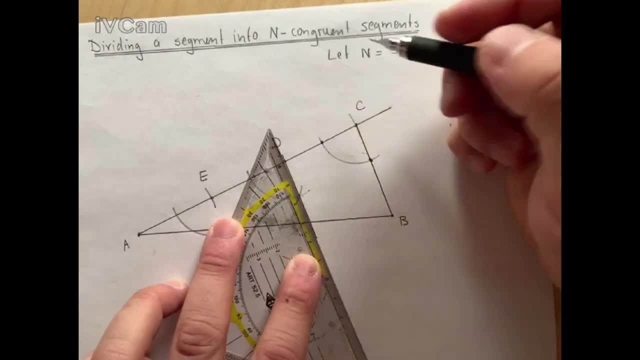 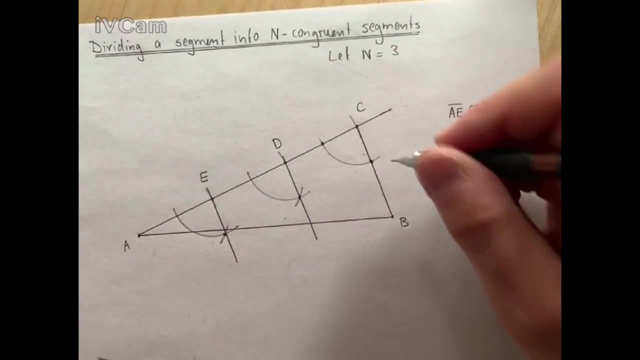 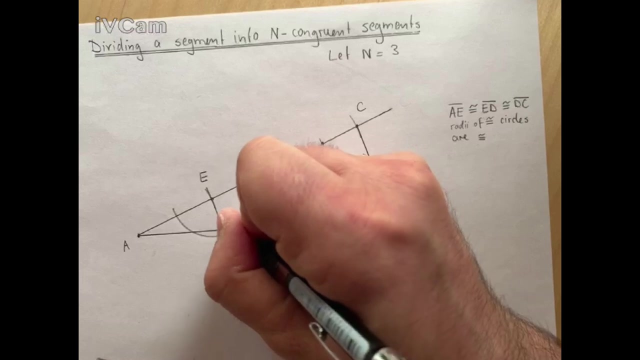 first we did this. this is step number two. okay, i i know i'm not writing things in order here, but it doesn't matter, because now we're talking about step number three here, okay, so why is that true? because there's actually a theorem that we have learned um in this unit here, basically, if we have, uh, two or more lines, they cut off congruent segments in one transversal, then they cut off congruent segments in every transversal and in order to see this better, you can actually turn the picture like this and say: you know what? that's the given. we know that this transversal is being cut by these lines that are parallel. therefore, every transversal that we draw must they have to have also congruent segments. so the reason for that will be the following, so let's write this in here: if, um, in this case we have three parallel lines, 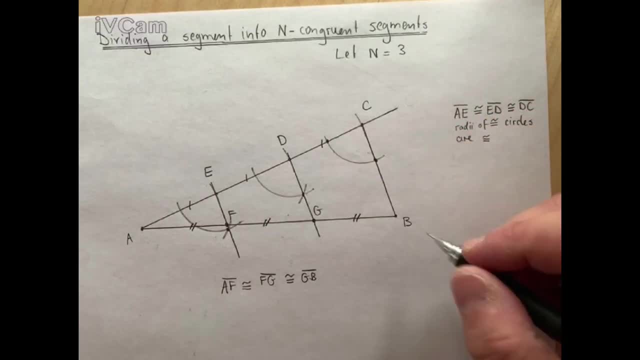 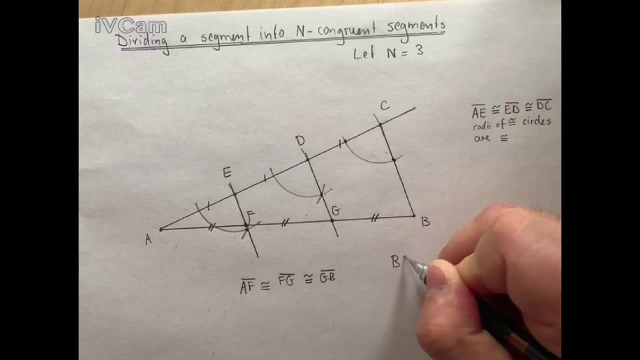 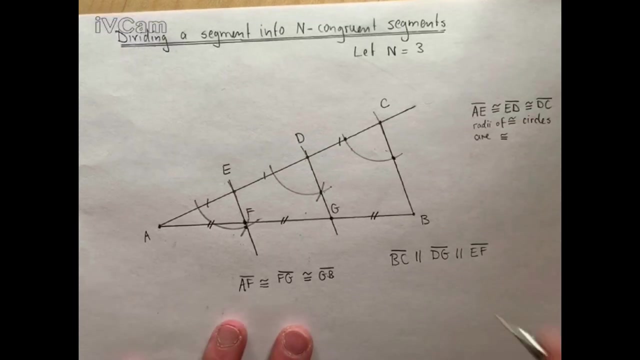 or we can say: if two or more parallel lines cut congruent segments in one transversal, then they cut off, then they cut or cut off, it doesn't matter. then they cut congruent segments in every transversal. okay, and that's basically the reason, okay, so first of all again, 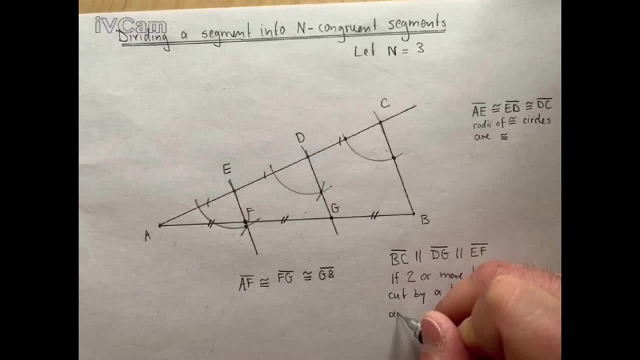 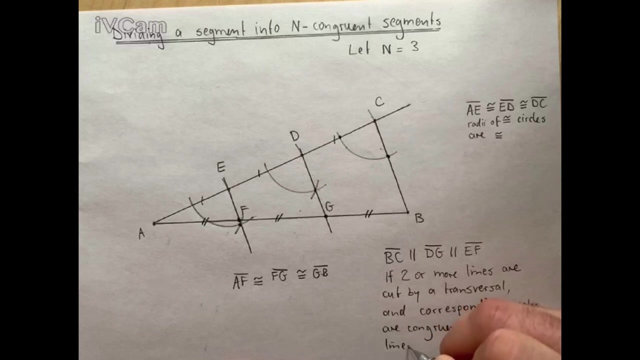 we made them congruent because of the compass rate of congruent segments. the circles are congruent. second step: we made the lines parallel because we used the copy angle method. so basically these are all the corresponding angles. they're congruent. then these three parallel lines cut off congruent segments in every transversal 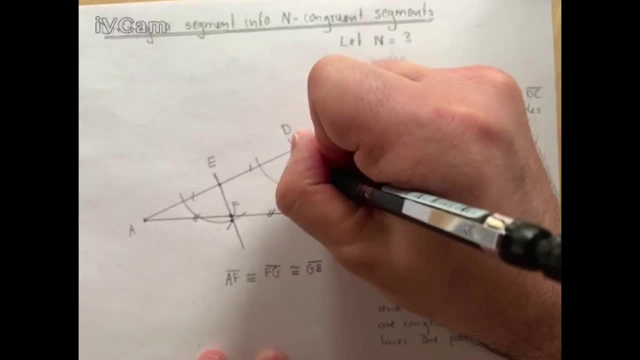 and that's basically it. okay, so that's how you construct this and that's how you justify this construction.